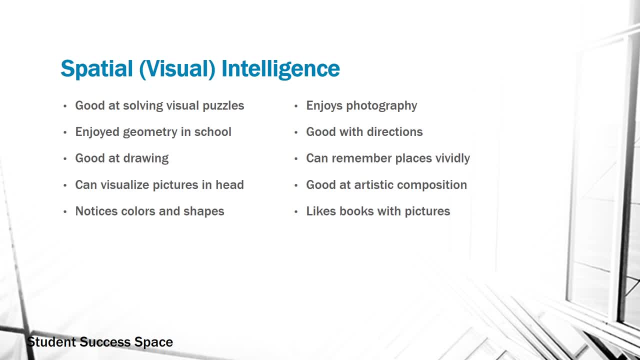 very aware of their surroundings, that they're able to place themselves within a 3D model. they're good at remembering images, they have a great sense of direction and they generally are going to learn best through drawings and visual aids. They're very good at solving problems, especially visual problems, and they tend to have enjoyed. 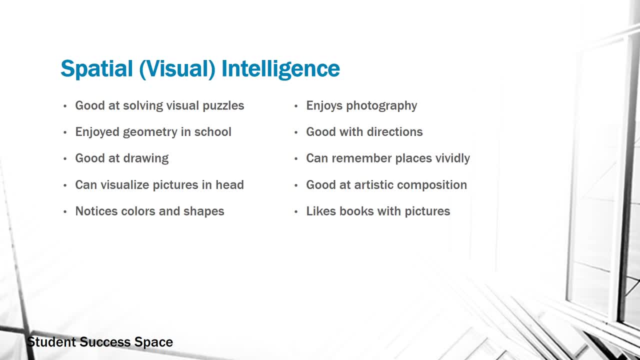 geometry in school. They're good at drawing. they can visualize pictures and they have a great ability to notice those colors as well as shapes. They may enjoy photography. they're good with directions and they have a very innate ability to remember places very vividly, with great detail. They're good at artistic composition and they 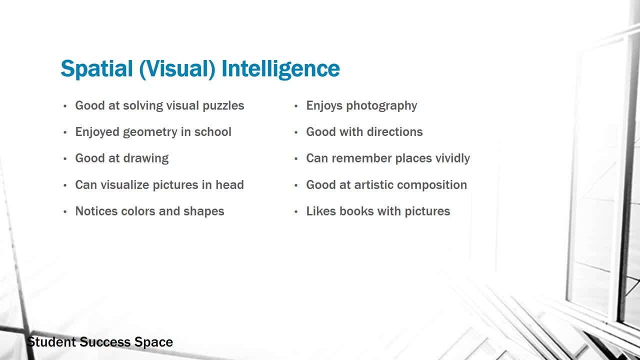 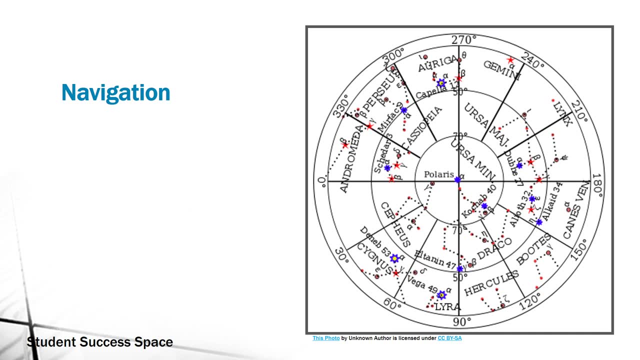 generally are going to like books that have many pictures within them. So some popular ways that we can use that spatial intelligence is within navigation, and navigation around those Carolina islands in the South Seas is accomplished, or was accomplished rather, by native sailors without instruments. They use the position of 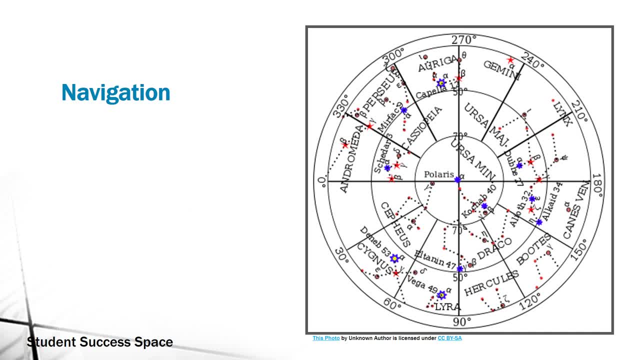 the stars as they viewed them from the various islands. They use weather patterns and water color as their principal signposts. The journeys were broken down into a series of segments and the navigator learned the position of the stars within each of those segments. And during the actual trip the navigator had to actually mentally picture a 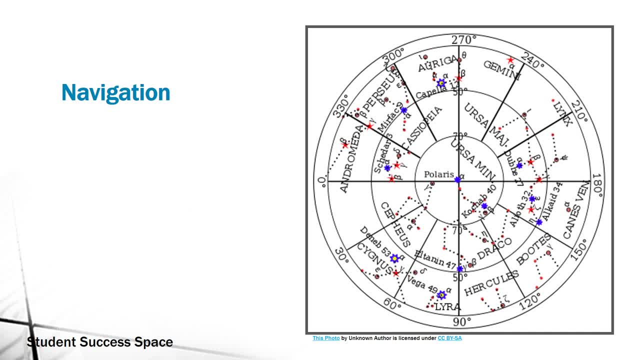 reference of the island as it passed under a particular star. So from the envisioning exercise he was able to compute the number of segments that were completed and the portion of the trip that remained. Any corrections that were made during the trip could be used as a reference to the 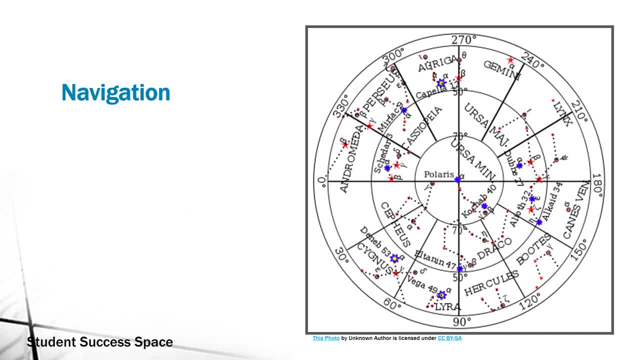 island. The direction and the heading that needed to be required was also an ability for him to be able to visualize. So the navigator could not see the islands as he was sailing along. Instead, he mapped locations within that 3D mental picture of his journey. 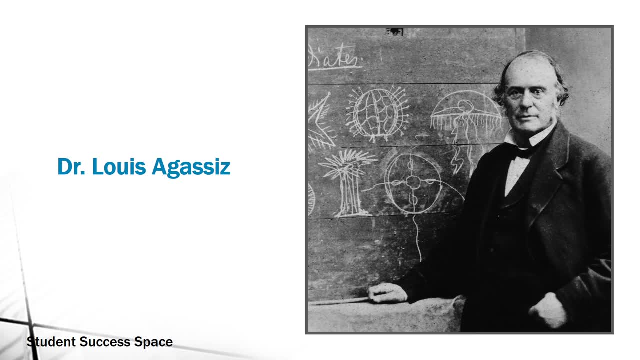 Another use of that spatial intelligence is Dr Louis Agassi. He's an American scientist and he valued detail. One day, a new assistant reported for duty and Agassi set the man to work, studying an unusual specimen of fish. Having given his instructions, he stepped out of the lab. 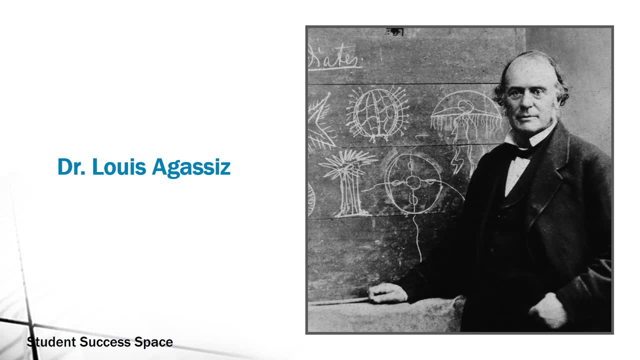 for what the assistant thought would be a few minutes. After half an hour of observation, the student felt that he really had discovered everything there was to know about that fish. But the scientist still did not return. Several more hours went by, during which the student was.